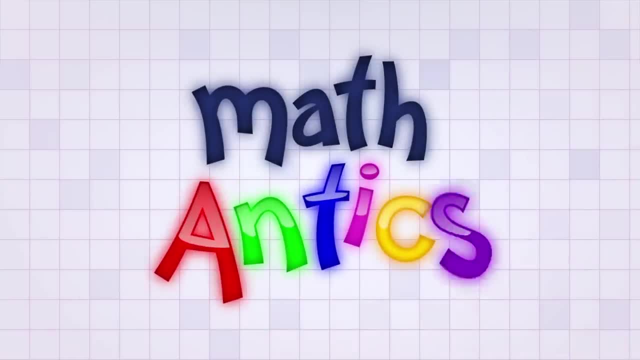 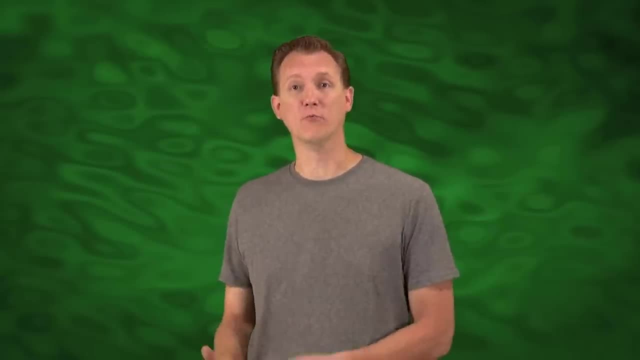 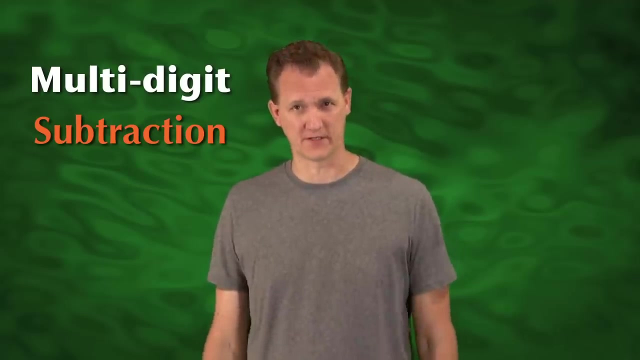 Hi and welcome to Math Antics. In this video we're going to learn how to do multi-digit subtraction. It's similar to doing multi-digit addition, like we learned in our last video, but there's a few important differences. The main difference is, with subtraction, the order of the problem matters. 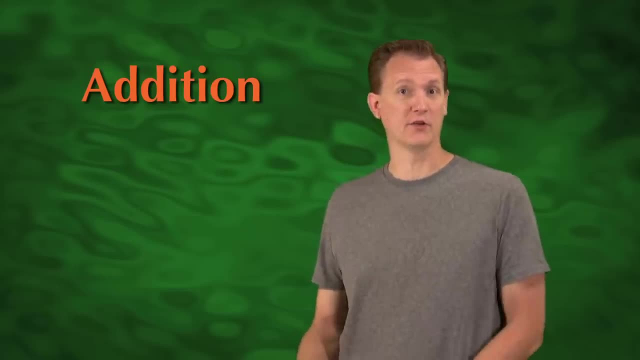 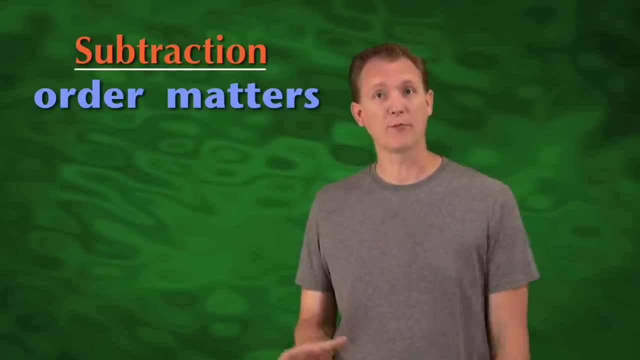 With addition you can switch the order of the numbers you're adding and you'll still get the same answer: 5 plus 2 equals 7 and 2 plus 5 equals 7.. But with subtraction, if you have the problem 5 minus 2, you'll get 3, but you can't switch the problem around. You won't get the same. 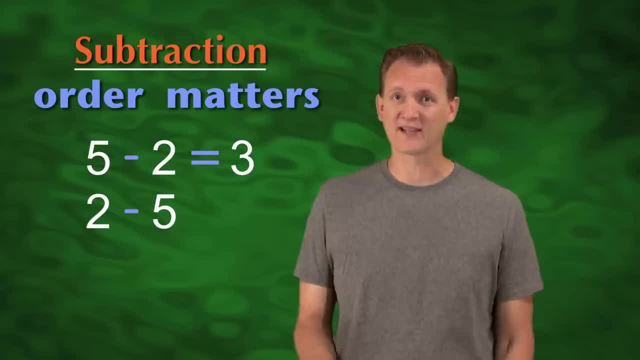 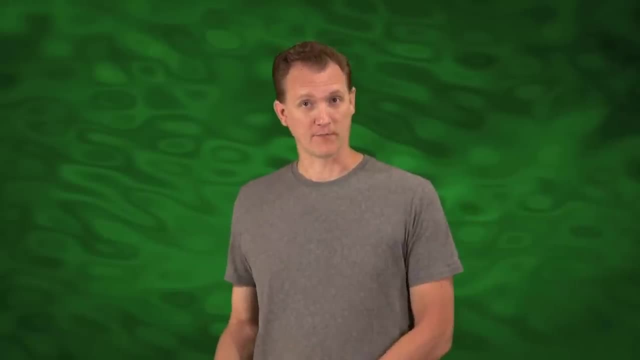 answer. if you try to do 2 minus 5 instead, In fact, you'll probably get confused because you'll be trying to subtract a bigger number from a smaller one. With multi-digit subtraction. it's important to remember that order matters, especially when you're rewriting your problem. Often you'll be given a project that is functionally rowed, suitable to each letter, and you're right, because you'll be trying to subtract a bigger number from a smaller one With multi-digit subtraction. it's important to remember that order matters, Especially when you're rewriting your problem. Often you'll be given a project. 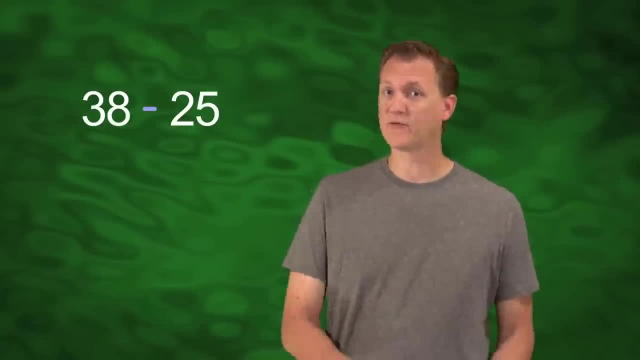 problem like this- 38 minus 25, and you'll have to rewrite it with the numbers stacked up, like we did with addition. But you have to make sure that the first number, the one you're taking from, goes on top and the number you're taking away is on the bottom. 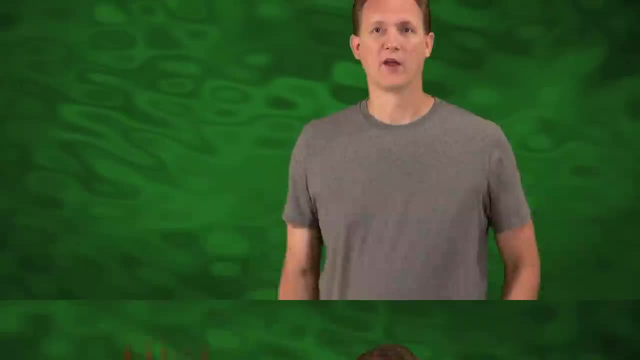 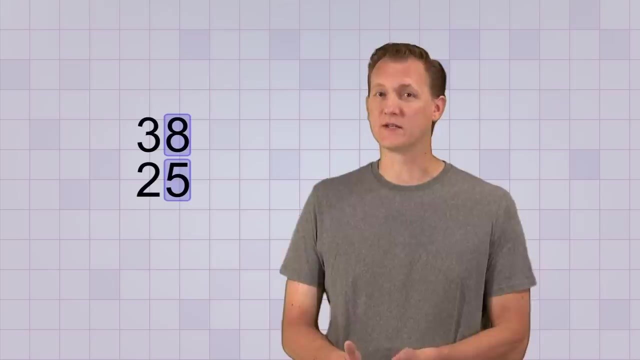 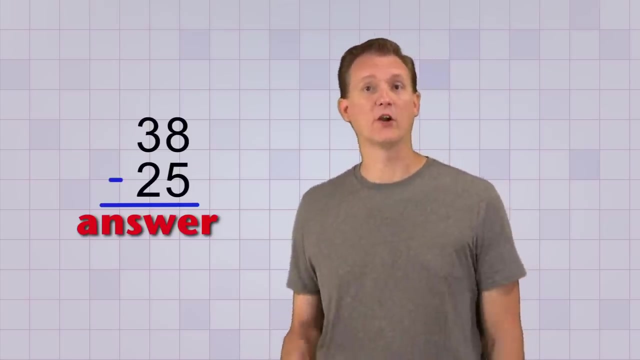 Another hint is that the bigger number should always be on top. Okay, let's go ahead and try this problem. We've got 38 on top and 25 below it, and the ones places are lined up just like they should be. Now we draw our line, so our answer can go below it, and we write a minus sign over here. 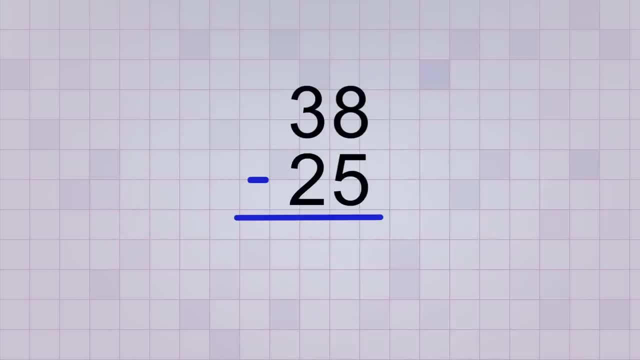 on the left to show that we're subtracting. Now we can start getting our answer and, just like with addition, we always start with the ones place column. Here we subtract the bottom number from the top. 8 minus 5 equals 3, so the 3 goes in the ones place of our answer. 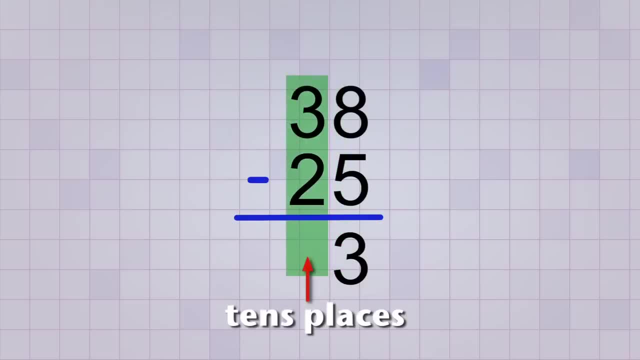 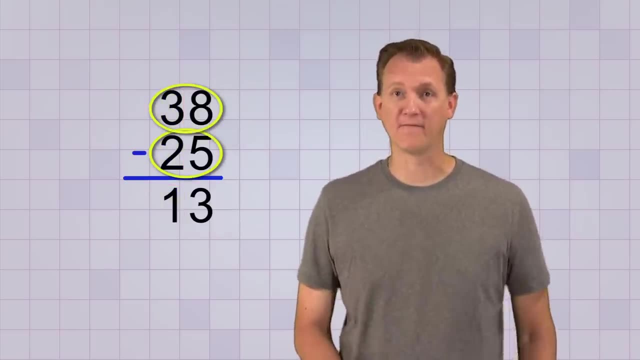 Now we move to the next place column to the left, the tens place. There we have 3 minus 2, which is 1.. There we just subtracted 25 from 38 and found out that the difference is 13.. 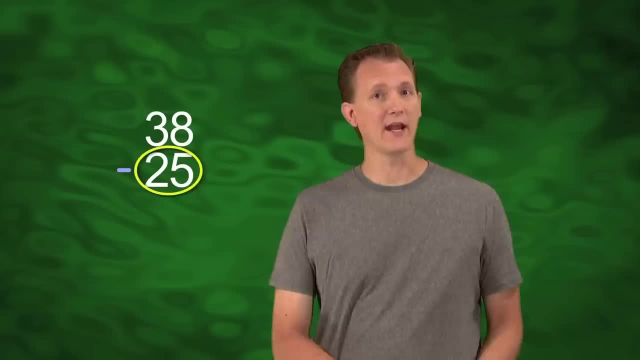 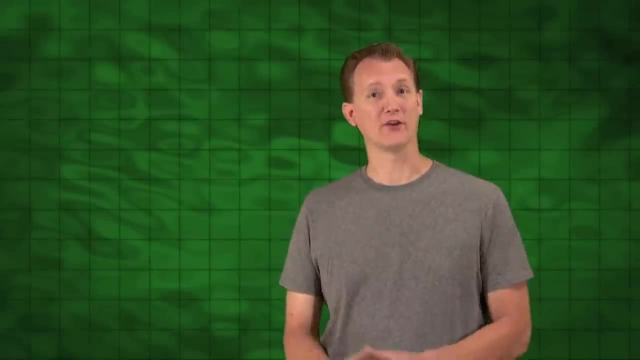 you're taking from goes on top and the number you're taking away is on the bottom. Another hint is that the bigger number should always be on top. Okay, let's go ahead and try this problem. We've got 38 on top and 25 below it, and 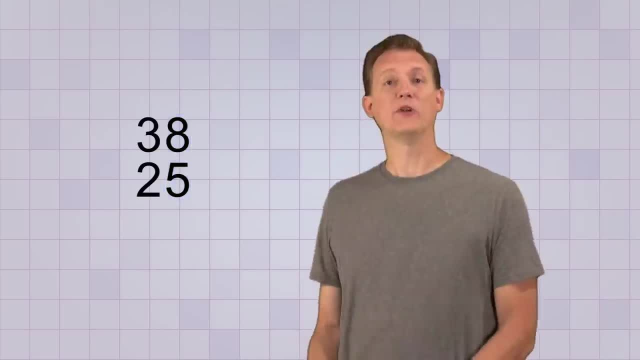 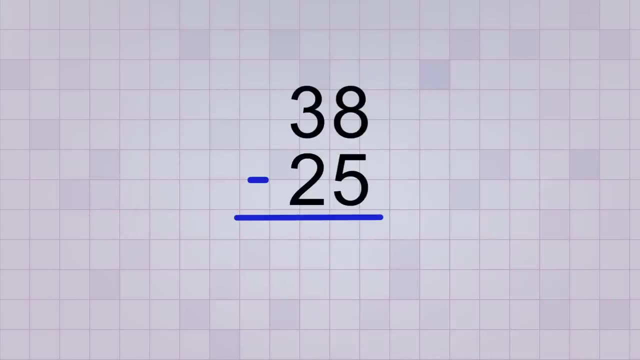 the ones places are lined up just like they should be. Now we draw our line, so our answer can go below it, and we write a minus sign over here on the left to show that we're subtracting. Now we can start getting our answer and just 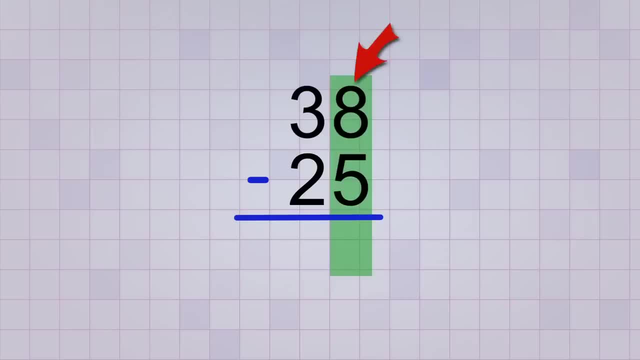 like with addition, we always start with the ones place column. Here we subtract the bottom number from the top. 8 minus 5 equals 3, so the 3 goes in the ones place of our answer. Now we move to the next place column, to the left, the tens place. There we have 3 minus. 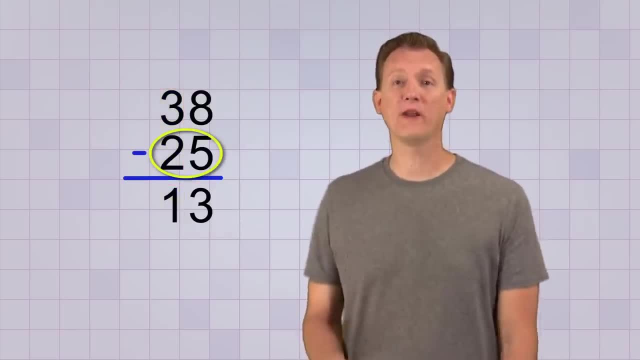 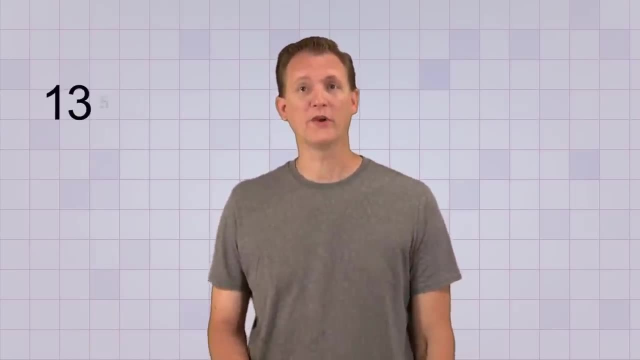 2,, which is 1.. There we just subtracted 25 from 38 and found out that the difference is 13.. Alright, let's see another example: 135 minus 27.. Aha, This is where multi-digit subtraction. 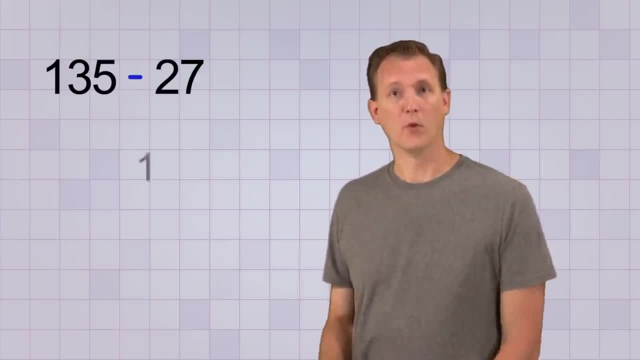 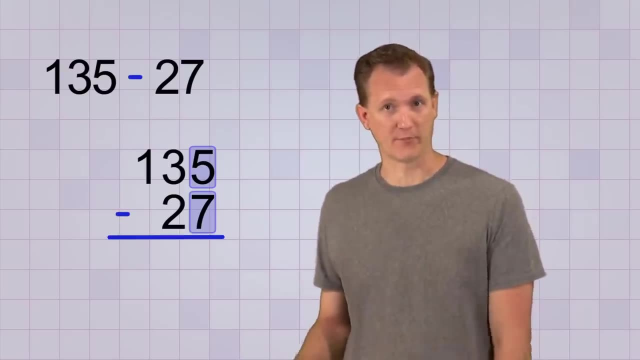 can get a little tricky. Let's rewrite our problem 135 on top, 27 below it, with the ones places lined up neatly and our answer line and subtraction symbol in place There. now we can start subtracting. Uh oh. 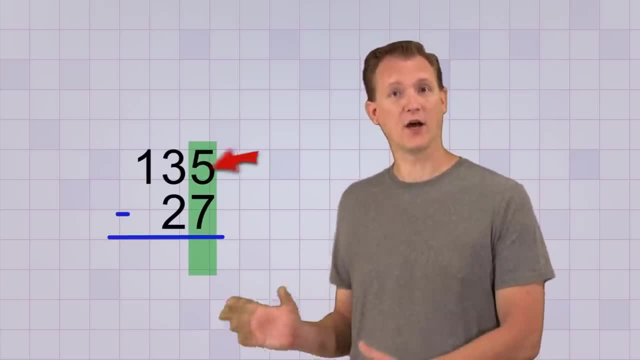 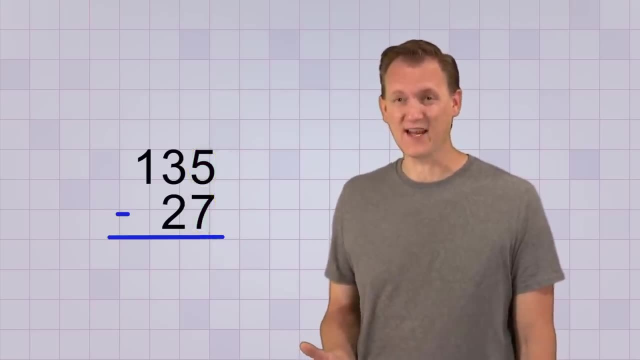 Look at this: In our ones place column, the digit on top is smaller than the digit on the bottom. How can we subtract a bigger digit from a smaller one? Did we make some kind of mistake? No, we wrote our problem correctly. The bigger number is on top. Sometimes this 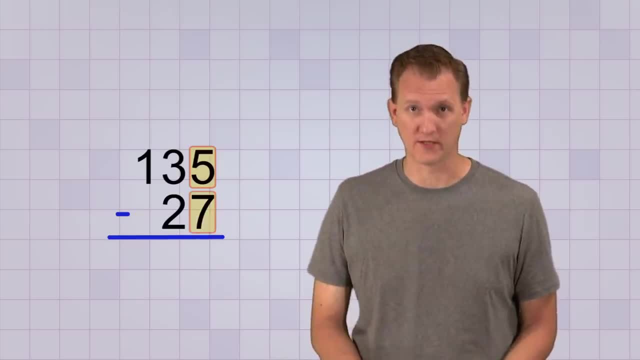 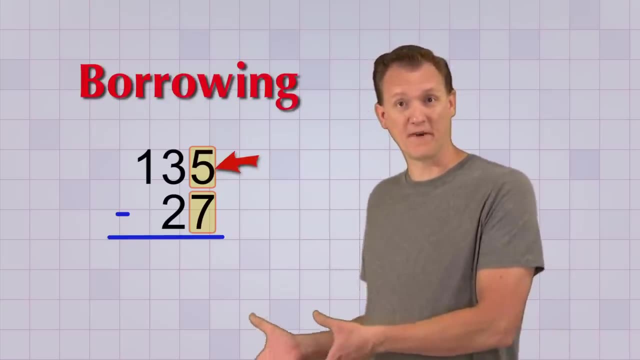 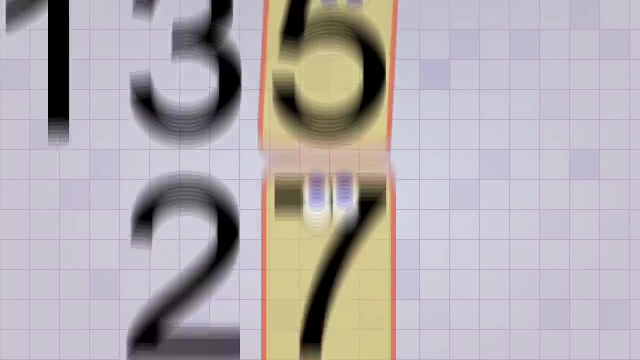 just happens, The top digit might be smaller than the bottom digit, so you can't subtract it, Unless you borrow. Here's how borrowing works. The top digit is 5, but the digit below it wants to take 7 away. Sorry, I don't have 7.. I only have 5.. 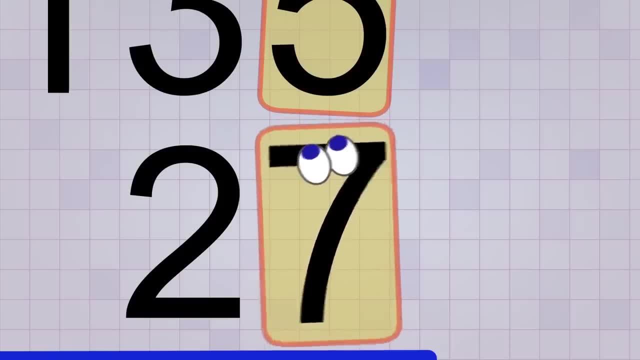 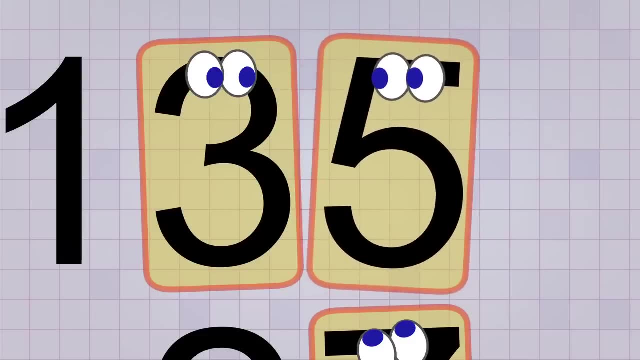 Well, what about your neighbor? He's in a bigger number place, He's loaded, So you can just borrow from him. Excuse me, I've got a little problem. Do you happen to have something I could borrow? Why, of course, Here you go. 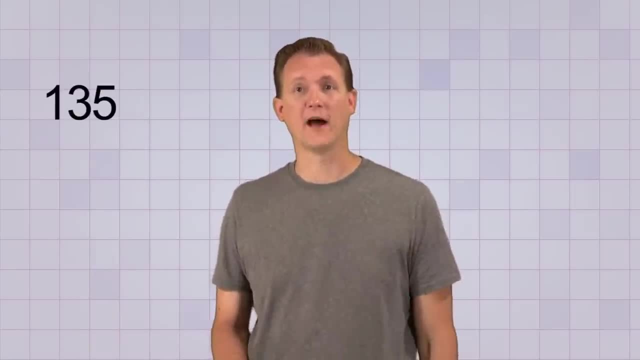 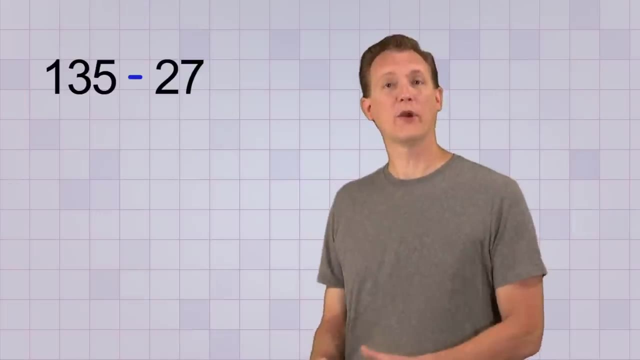 Alright, let's see another example: 135 minus 27.. Aha, This is where multi-digit subtraction can get a little tricky. Let's rewrite our problem: 135 on top, 27 below it, with the ones places lined up neatly. 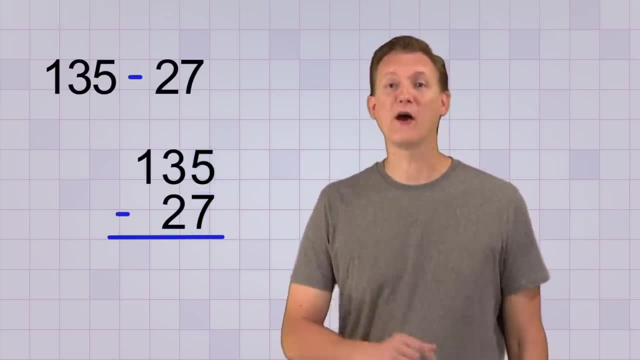 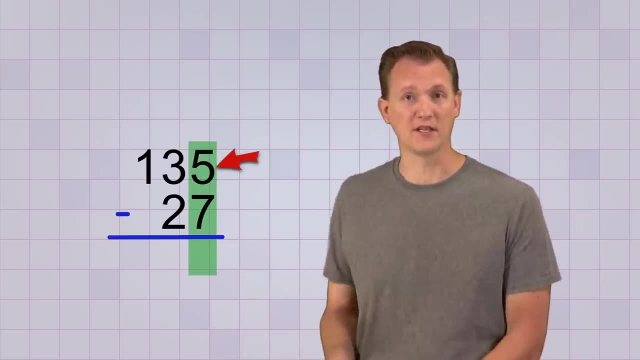 and our answer line and subtraction symbol in place There. now we can start subtracting. Uh oh, Look at this. In our ones place column, the digit on top is smaller than the digit on the bottom. How can we subtract a bigger digit from a smaller one? Did we make some kind? 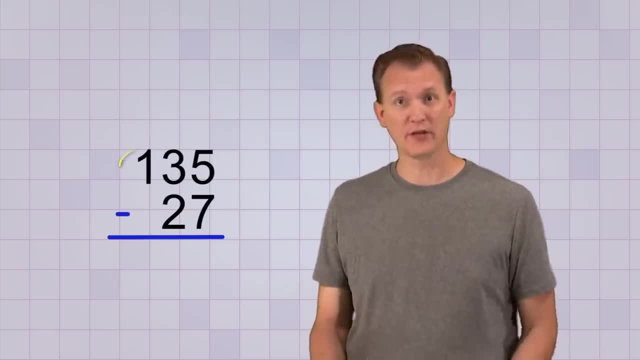 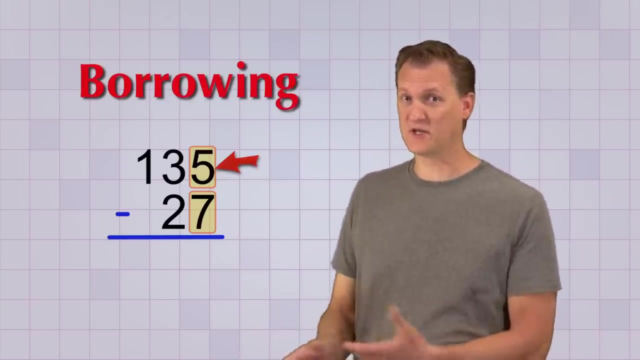 of mistake. No, we wrote our problem correctly. The bigger number is on top. Sometimes this just happens The top digit might be smaller than the bottom digit, so you can't subtract it Unless you borrow. Here's how borrowing works. The top digit is 5, but the digit below it wants to take. 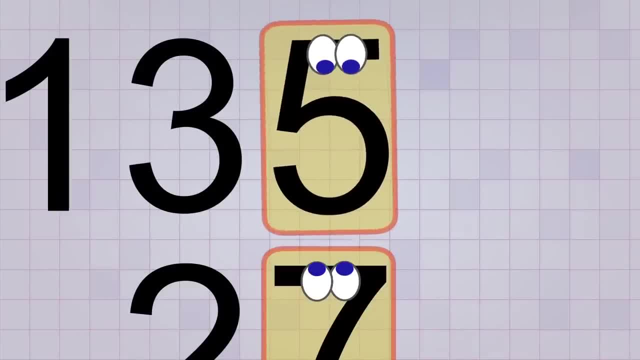 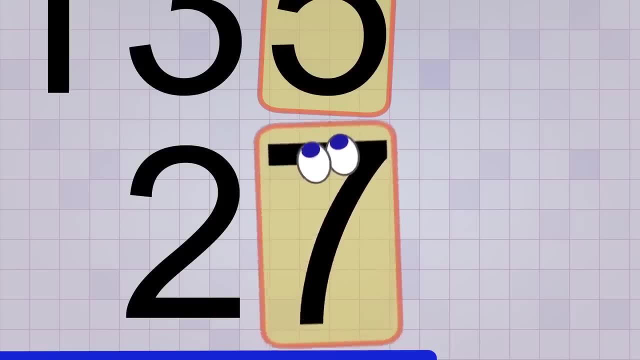 7 away. Sorry, I don't have 7.. I only have 5.. Well, what about your neighbor? He's in a bigger number place. He's loaded, So you can just borrow from him. Excuse me, I've got a little problem. Do you happen to have something I could borrow? 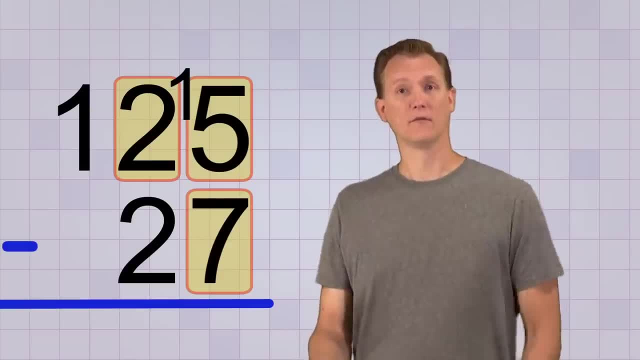 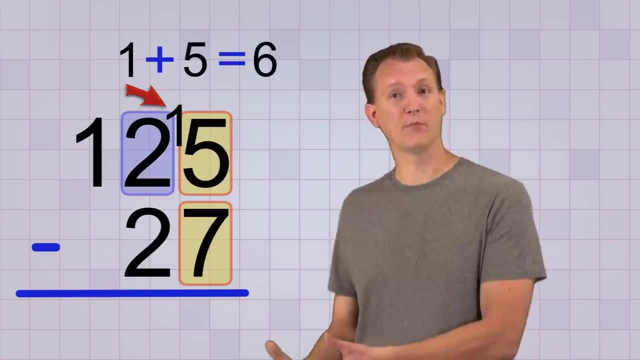 Why? of course, Here you go. Great, That 1 will help, But if you just add 1 to 5, you'd get 6.. But fortunately this 1 came from the next number place and it really represents a 10.. And when we add 10, 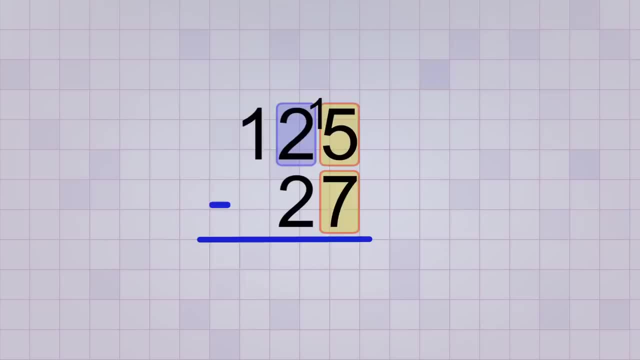 to 5, we get 15,, which is big enough. Now, instead of this column being 5 minus 7, it's 15 minus 7.. And 15 minus 7 equals 8.. Okay, we've got the first digit of our answer. Now we can move on to the next column. But 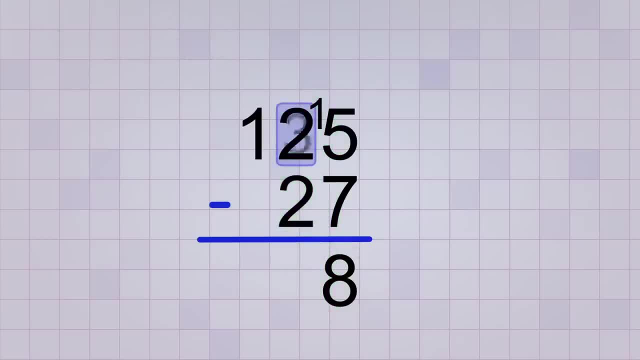 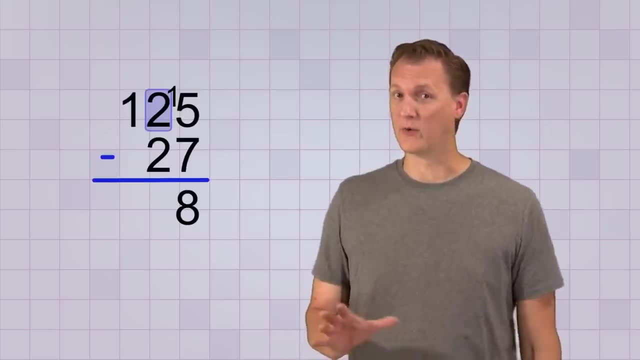 remember we borrowed from that number place. It used to be a 3,, but now it's a 2.. It went down by 1 because we borrowed from it. Well, remember we really borrowed 10 because it was in the next number place. 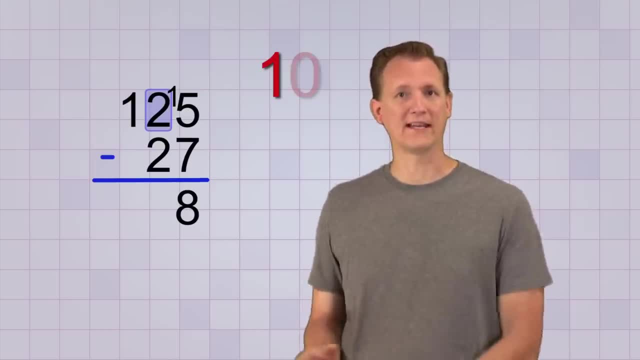 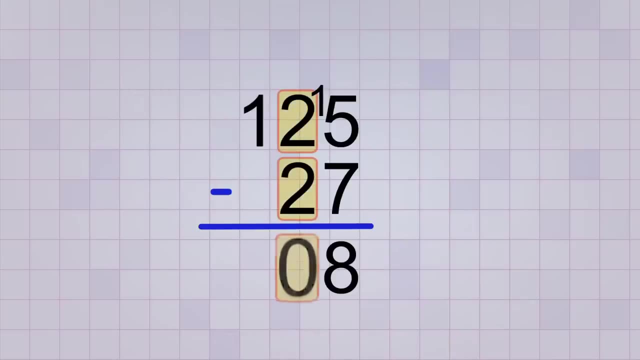 But it's sometimes easier to just think of it as borrowing a 1, and getting to stick that 1 in front of the digit that needed to borrow. So in the tens place we have 2 minus 2, which gives us 0 in our answer. And then our last. 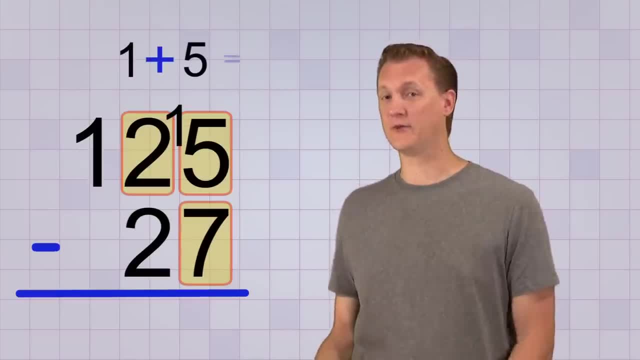 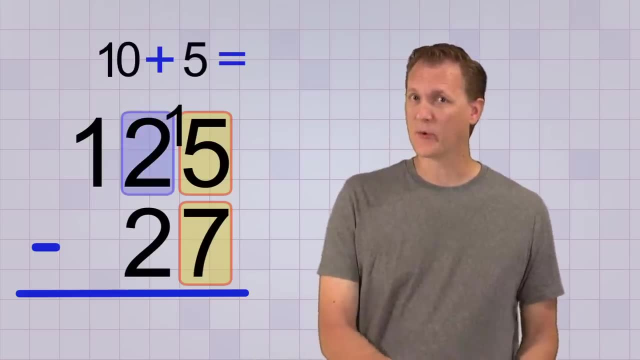 Great, That 1 will help, But if you just add 1 to 5, you'd get 6.. But fortunately this 1 came from the next number place and it really represents a 10.. And when we add 10, 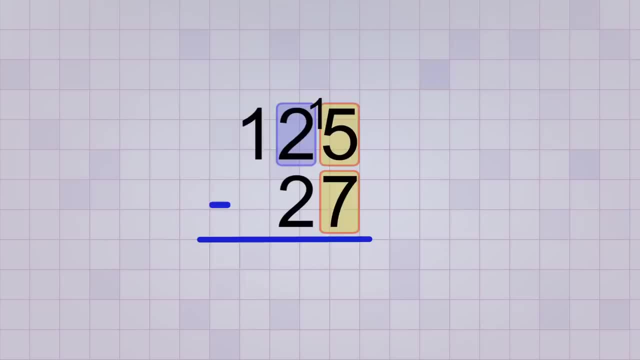 to 5, we get 15,, which is big enough. Now, instead of this column being 5 minus 7, it's 15 minus 7.. And 15 minus 7 equals 8.. Okay, we've got the first digit of our answer. Now we can move on to the next column. But 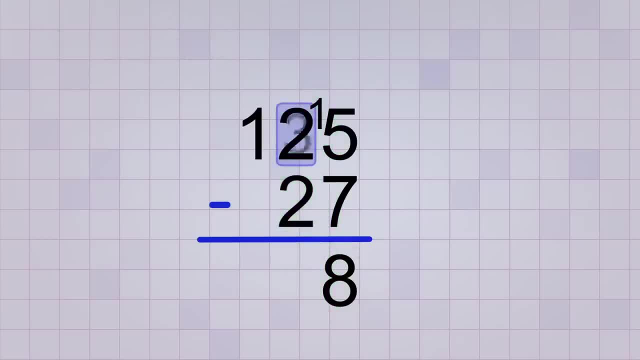 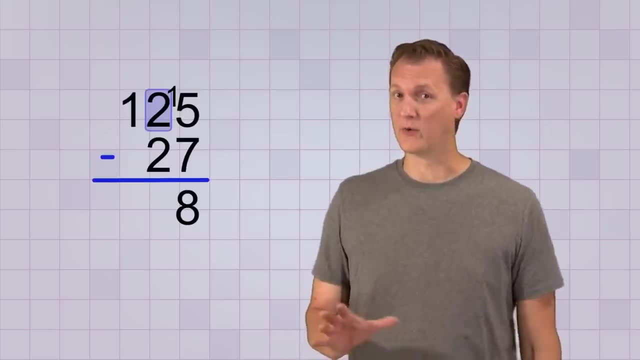 remember we borrowed from that number place. It used to be a 3,, but now it's a 2.. It went down by 1 because we borrowed from it. Well, remember we really borrowed 10 because it was in the next number place. 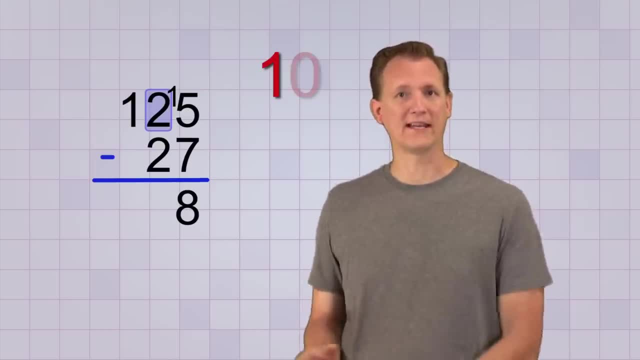 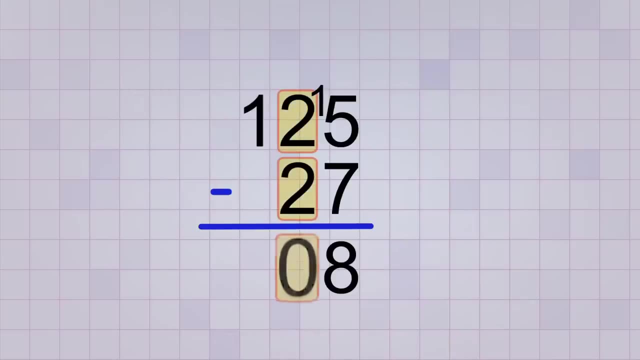 But it's sometimes easier to just think of it as borrowing a 1, and getting to stick that 1 in front of the digit that needed to borrow. So in the tens place we have 2 minus 2, which gives a 0 in our answer And then our last. 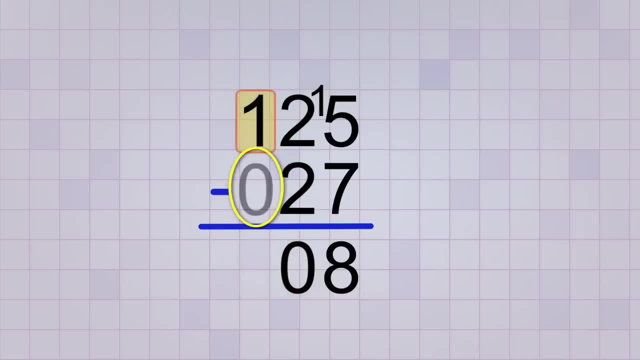 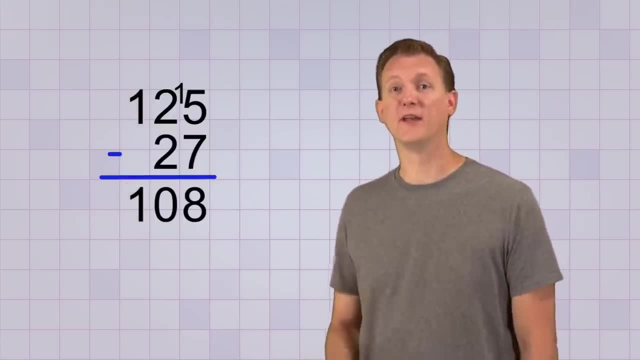 column just has 1 minus nothing or 1 minus 0, so that's still just 1.. There We've calculated that the difference between 135 and 27 is 108.. Alright, let's try another example with borrowing Or regrouping a number. 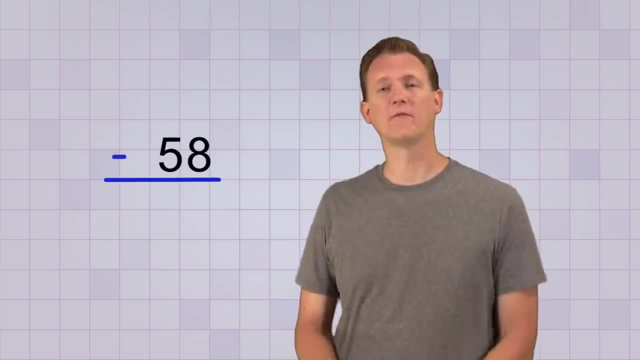 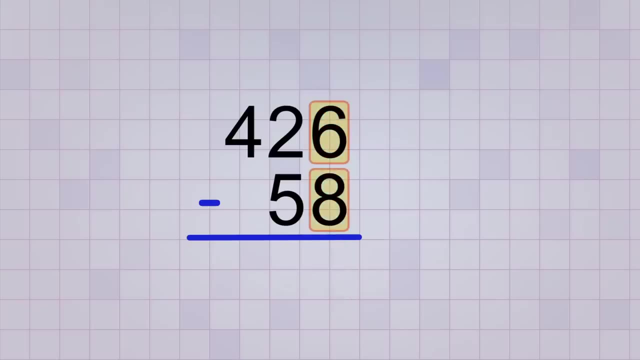 Regrouping, as some teachers call it. Let's subtract 58 from 426.. Again, we start by subtracting the digits in the ones place column. Here we have 6 minus 8.. And since 6 is too small to subtract 8 from, we'll need to borrow. 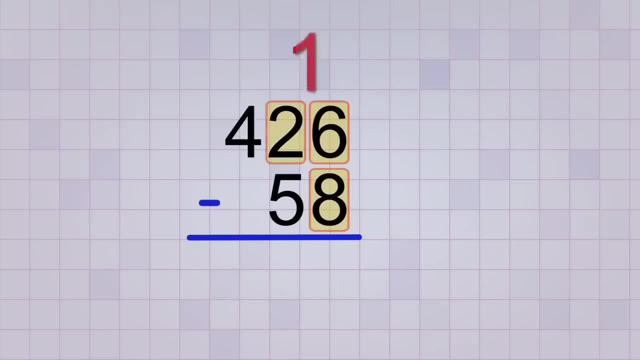 We always borrow from the number place on the left. We'll borrow a 1,, which is really a 10, and we'll write it in front of our borrowing digit, in this case 6,, which gives us 16.. And don't forget to make the digit we borrowed from smaller by 1.. 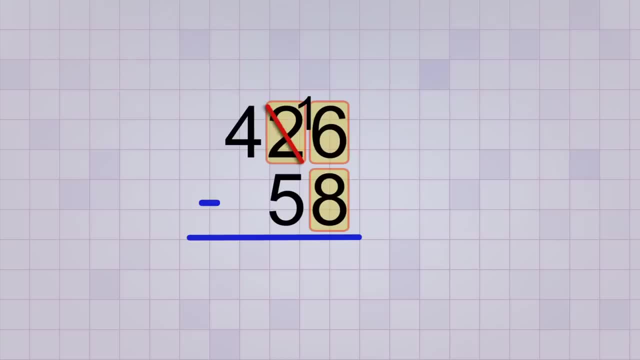 We'll write it in front of our borrowing digit, in this case 6,, which gives us 16.. And don't forget to make the digit we borrowed from smaller by 1.. You can just cross it out and write the new smaller number above it like this: 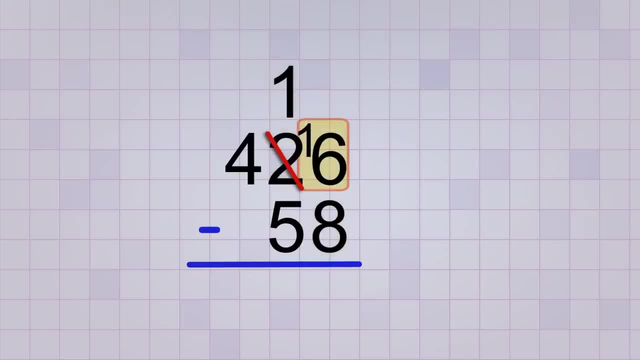 Okay, now we can subtract from the first column: 16 minus 8 equals 8.. Now for the tens place. Since we borrowed from this column, it's become 1 minus 5.. But again, the top number's too small, so we'll have to borrow again. 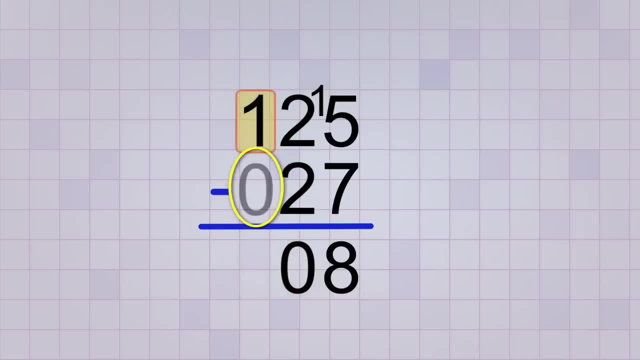 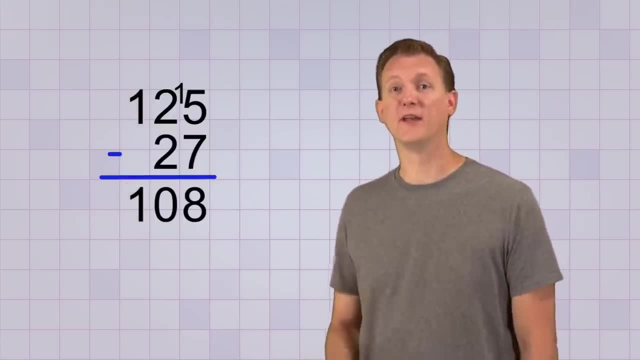 column just has 1 minus nothing or 1 minus 0, so that's still just 1.. There We've calculated that the difference between 135 and 27 is 108.. Alright, let's try another example with borrowing Or regrouping a number. 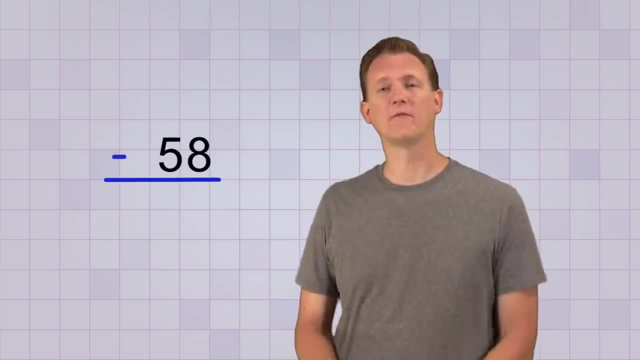 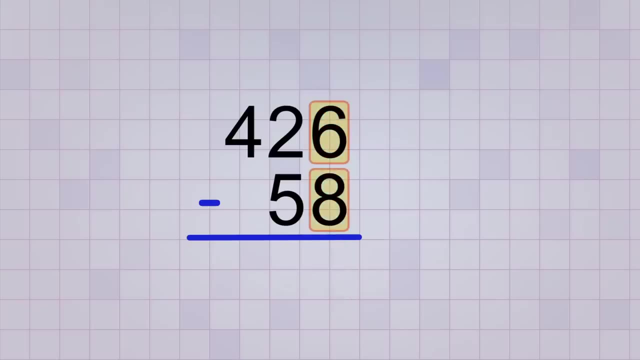 Regrouping, as some teachers call it. Let's subtract 58 from 426.. Again, we start by subtracting the digits in the ones place column. Here we have 6 minus 8.. And since 6 is too small to subtract 8 from, we'll need to borrow. 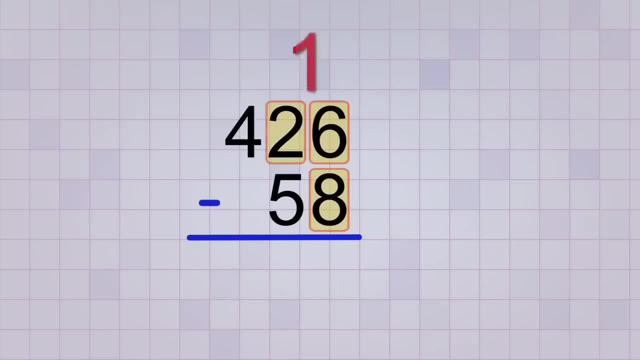 We always borrow from the number place on the left. We'll borrow a 1,, which is really a 10, and we'll write it in front of our borrowing digit, in this case 6,, which gives us 16.. And don't forget to make the digit we borrowed from smaller by 1.. 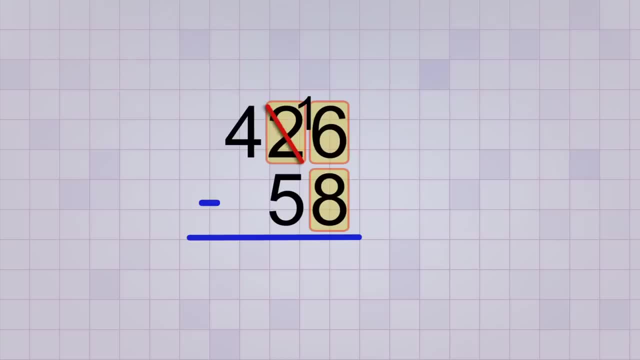 We'll write it in front of our borrowing digit, in this case 6,, which gives us 16.. And don't forget to make the digit we borrowed from smaller by 1.. You can just cross it out and write the new smaller number above it like this: 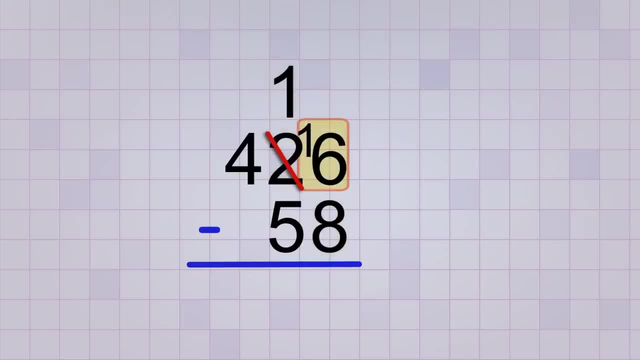 Okay, now we can subtract from the first column: 16 minus 8 equals 8.. Now for the tens place. Since we borrowed from this column, it's become 1 minus 5.. But again, the top number's too small, so we'll have to borrow again. 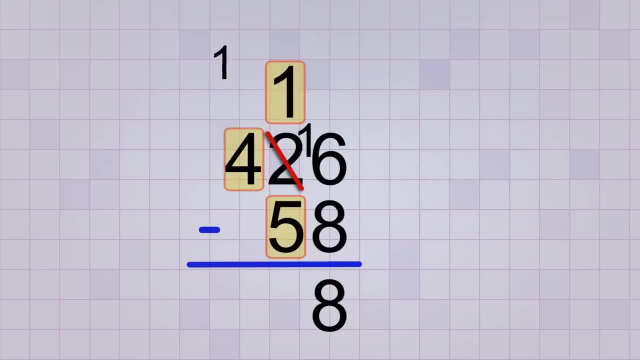 We borrow a 1 from the next number place over, which means that digit will change from a 4 to a 3.. Then we put the 1 in front of the borrowing digit, in this case 6.. But again the top number's too small, so we'll have to borrow again. 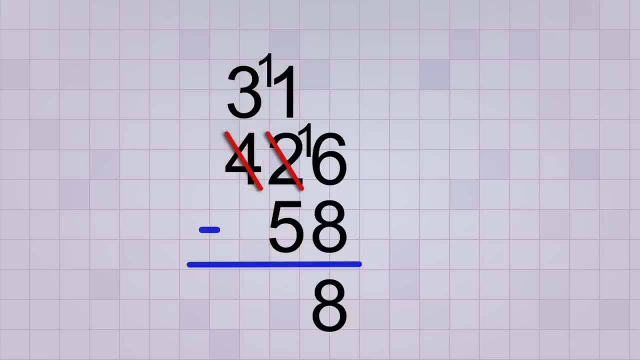 And again the top number's too small so we'll have to borrow again. Then we put the 1 in front of the borrowing digit, in this case 6.. Now we can do the subtraction for that column: 11 minus 5 equals 6.. 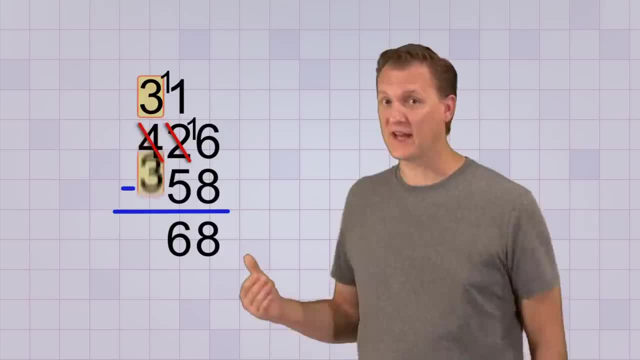 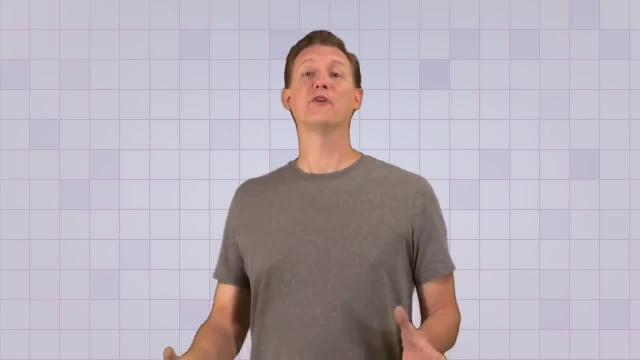 And the last column's easy. We bring that left over 3 down to the answer line because there's nothing there to subtract from it, And that means 368 is our answer. So now you know the basics of multi-digit subtraction. But before you move on to practicing with exercises, I want to show you one more important. 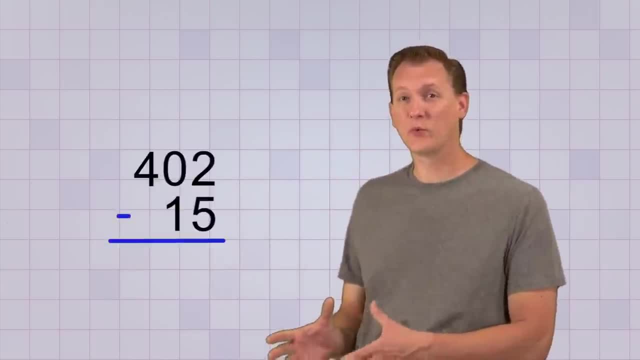 trick. Once in a while you'll come across a situation where you need to borrow from the next number place. Once in a while, you'll come across a situation where you need to borrow from the next number place, where you need to borrow from the next number place over, but that digit happens to be a zero.